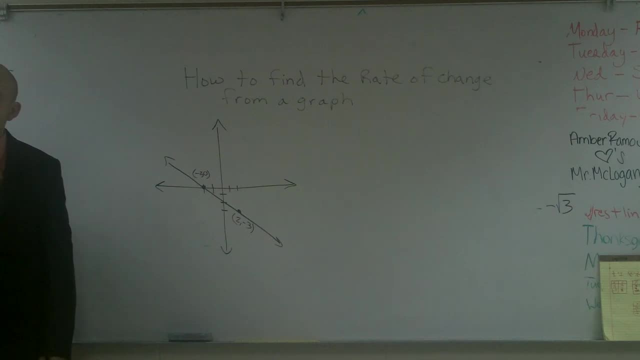 of rate of change is it's the ratio of the change in two quantities And we're talking about when you're dealing with a linear graph or at the table or between two points. our two quantities are going to be our x and y values, So what we call the rate of change. 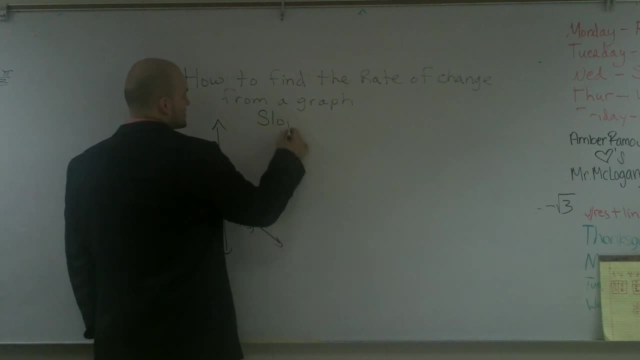 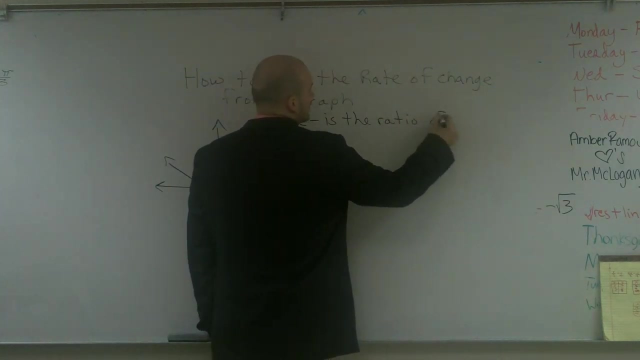 of x and y values is what we call our slope. I'm just going to write this down here: Slope is the ratio of the change in y values over x values. Now you might say: well, all right, Mr McGlogin, I have this line. and 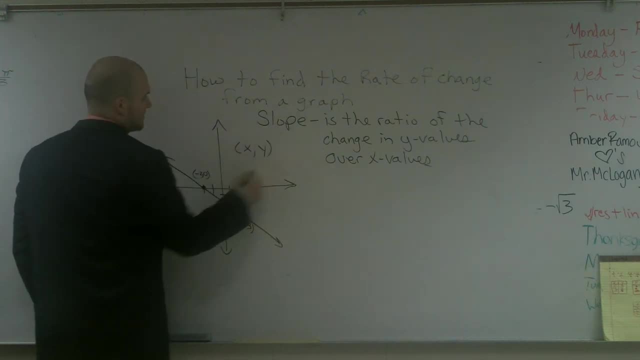 I have these two points. Well, remember, a point always comes in the form of x comma y. So here's: my x is negative 2, my y is 0.. Over here, x is 2, y is negative 3.. And the 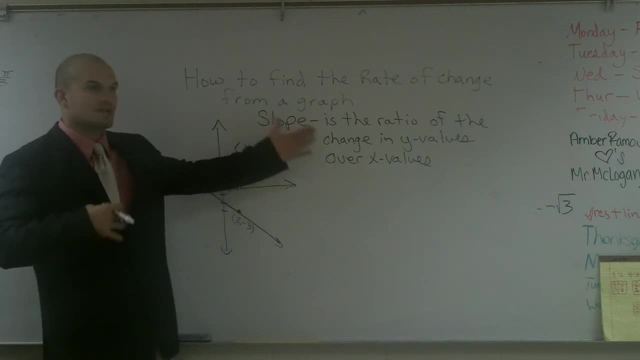 one example I like to keep on going through is: if they're talking about change, what do you mean by change? How do you calculate the change? Well, if I had $20 yesterday and I only have $2 today, what would I get? I'd get $2. 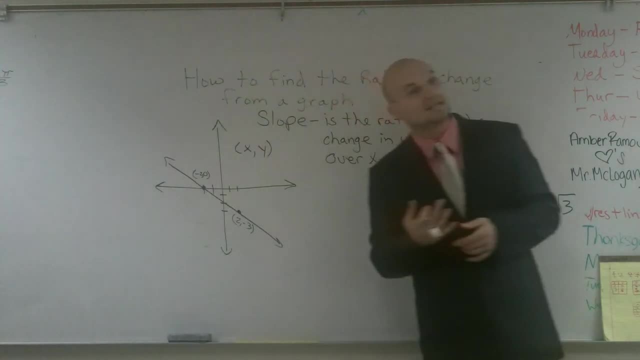 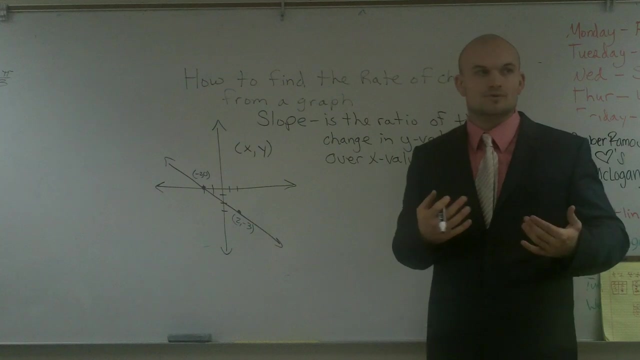 $2 is the change in the amount of money I have And the change in the amount of money I had was 18.. It would be, yes, I lost 18, so it would be a negative 18.. But the change what I did was I took how much money I had, which. 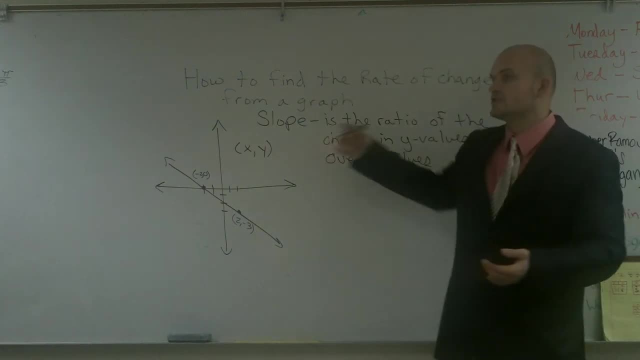 was 20, and I subtracted 2.. So when you're trying to find the change, you're finding the difference. OK, so you're always going to use subtraction. So I want to find the change in my y values, I need to subtract them. So I'm going to say: well, this y value 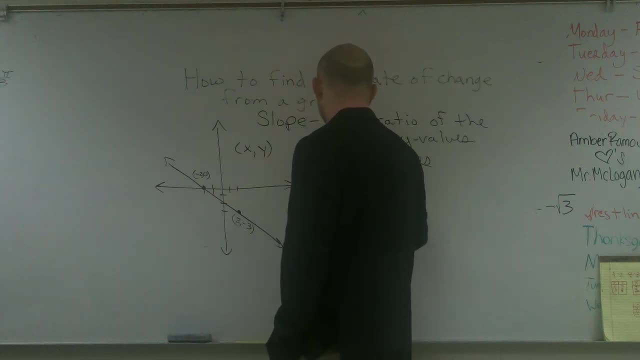 is 3, so I'm going to say slope, And we're going to get into the general formula for sloping this in a little bit. The general formula for this is going to be negative 3,, that's one y value minus my other. 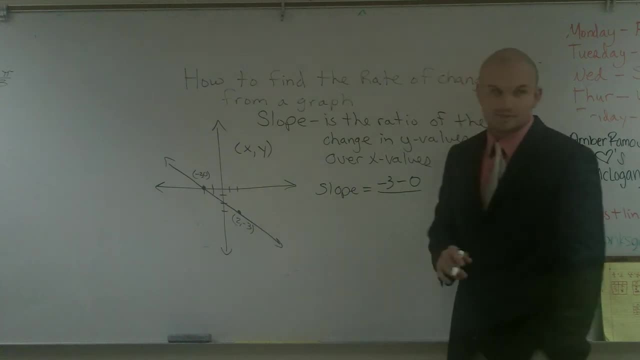 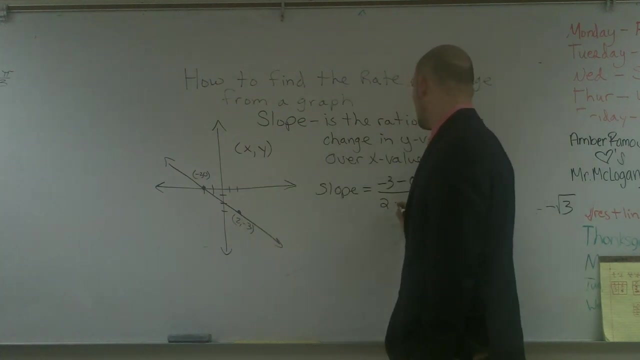 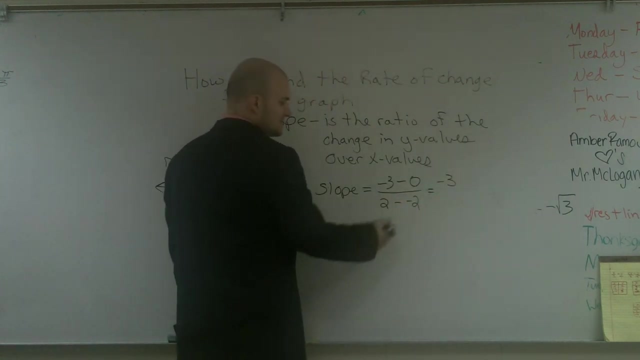 y value, which is 0, over the change in my x value, which is 2 minus negative 2.. Now one thing to notice is: negative 3 minus 0 is obviously going to be negative 3, and 2 minus negative 2,. those both become positive and we get 4..